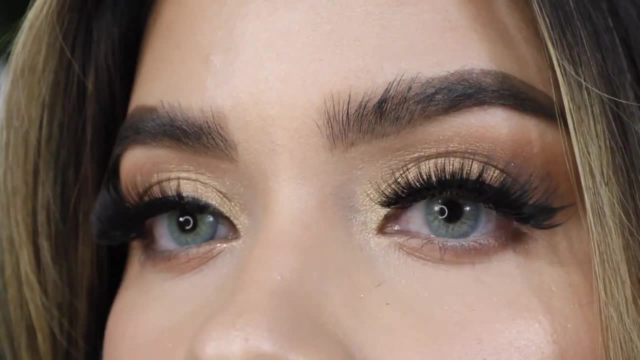 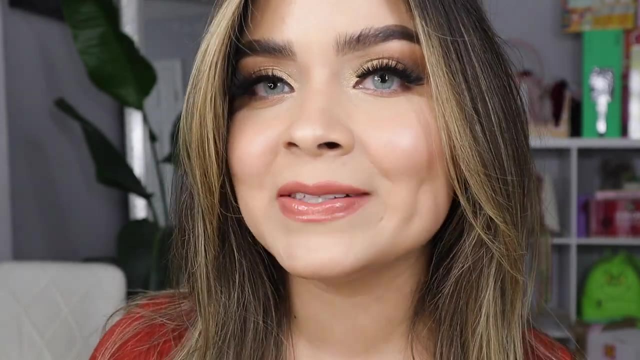 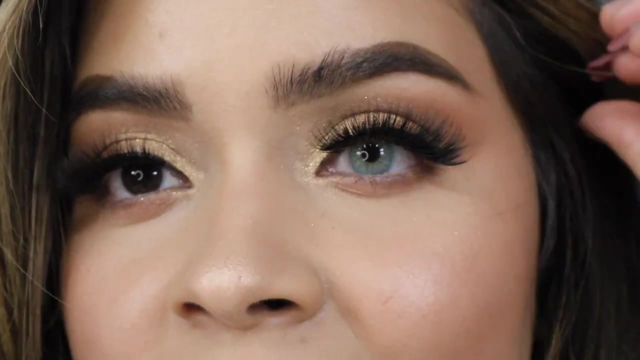 natural color and i was like: no, these are color contacts. so it was like shocking for them to me, for me to say that anyways, uh, this is how samba green looks on a dark brown contacts. samba green and this is my dark brown eye, as you can see this color, it is such a really beautiful natural. 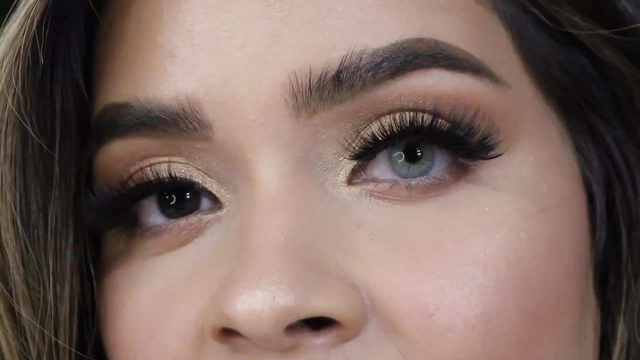 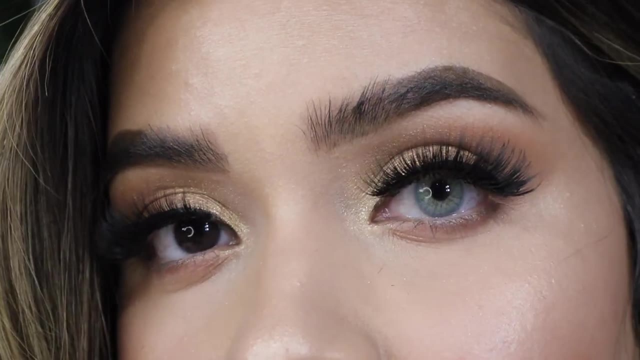 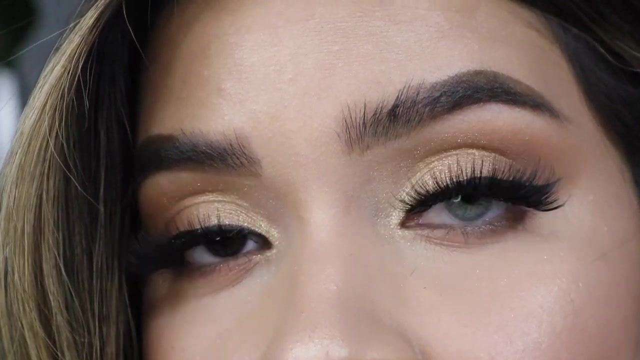 ocean blue color contact and this is from the aquarella collection quarterly. i just want to get out there that the collection from aquarella, if it is definitely a three month duration, but for me i had taken really good care of my color contacts and i do. 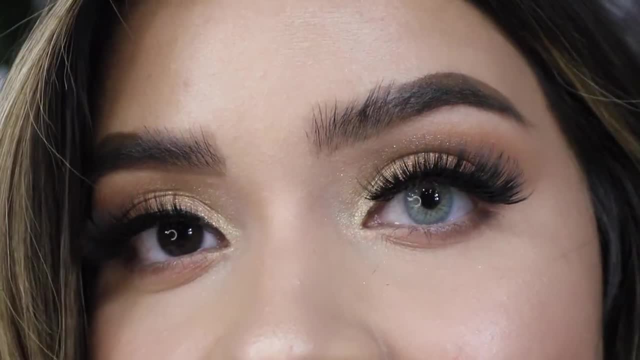 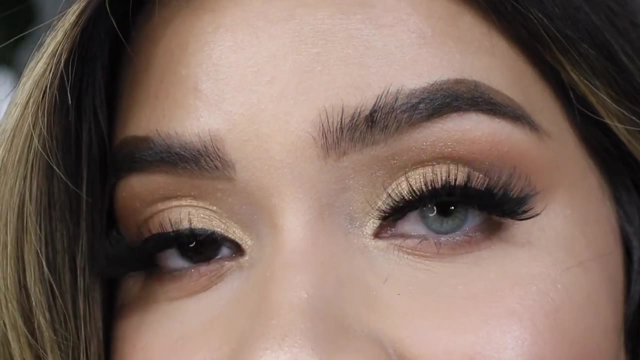 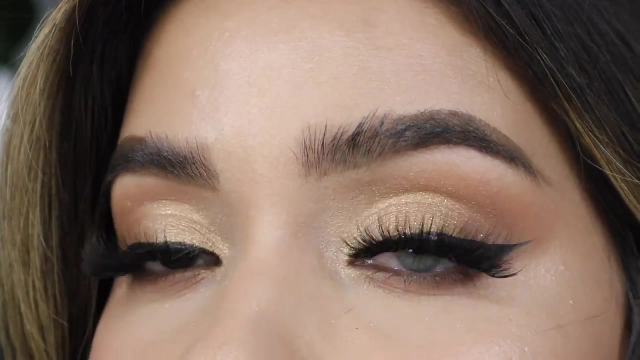 solution: clean, cleaning. so these color contacts have lasted me for about six months already. so it's insanely if you guys sanitize your color contacts. really good. color contact samba green: it has no limbering on it, which i really love whenever color contacts don't have no limbering. 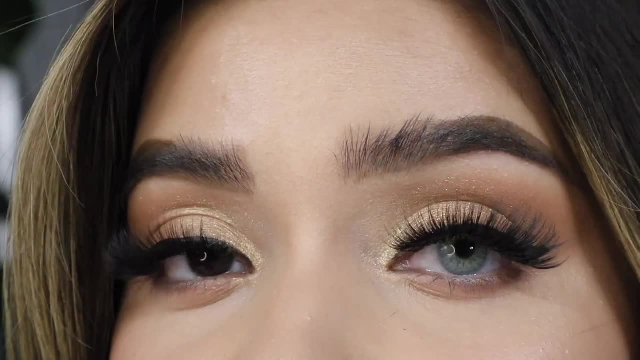 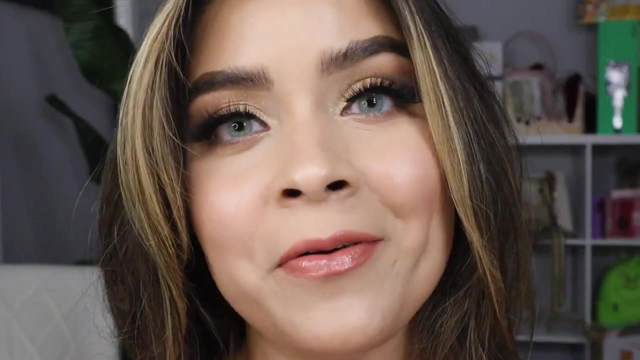 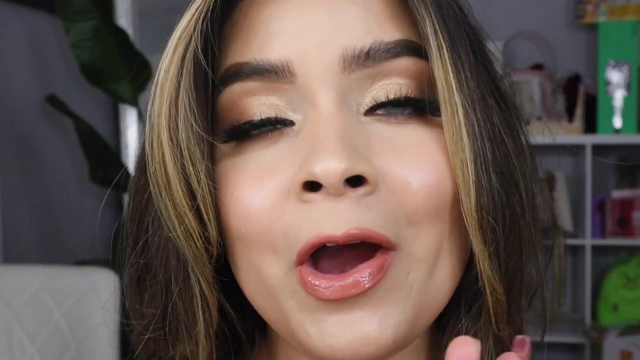 because it makes the color contact fade in so perfectly to a dark red eye and it makes it look super, super real. i already have the two different color contacts in my eyes. i'll take a minute for you guys to comment down below on which one you think is the samba green and which one you think. 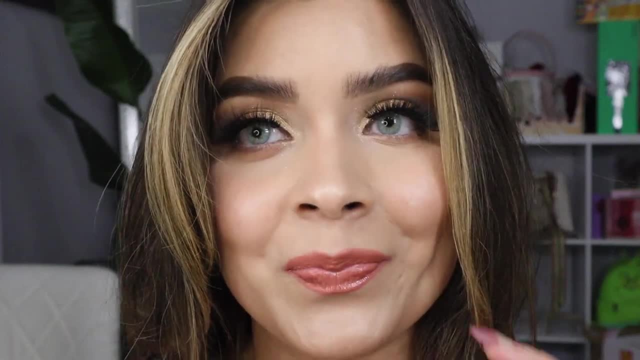 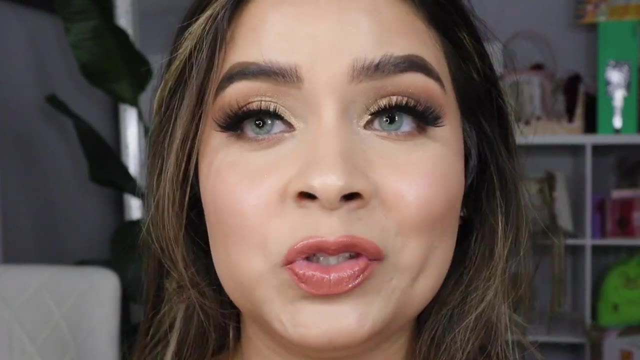 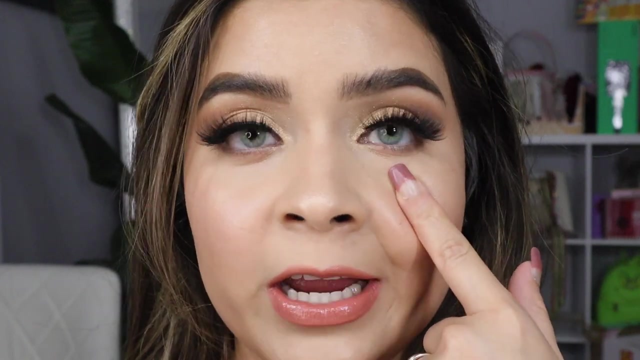 it's the hydrocore iponema. so both of these lenses- okay, let me get my hair back- both of these dense lenses look so. so they both look the same, but they're different. here i'm wearing the samba green and here i'm wearing the hydrocore rio iponema. 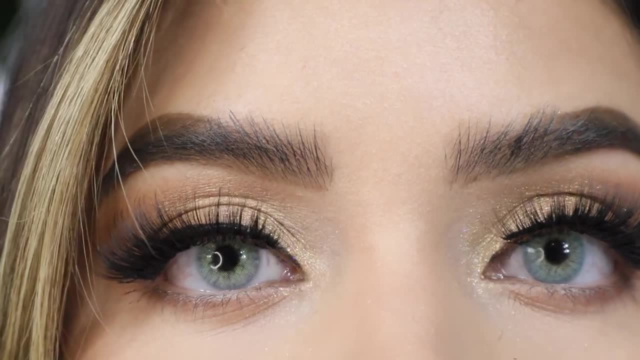 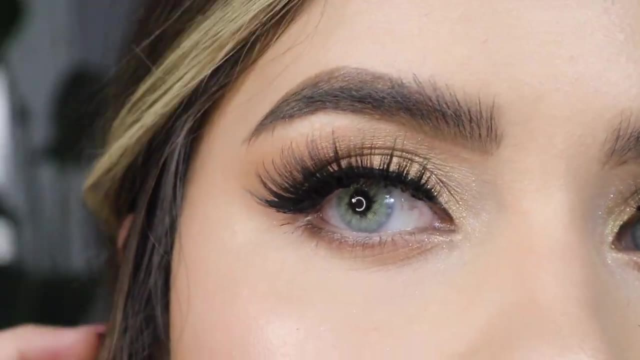 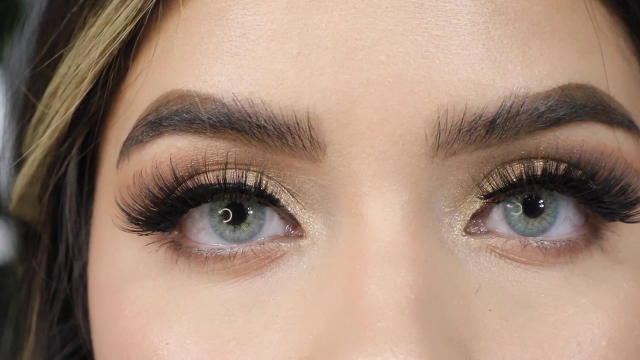 it is definitely both of them. looking at myself, they look so, so, so familiar. except for this one. i feel like it has more of a faded in dinner and i like how it looks. samba green is just looks so beautiful on dark red eyes. it looks really, really realistic because 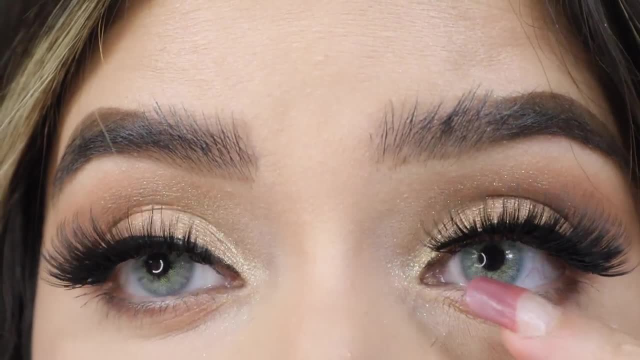 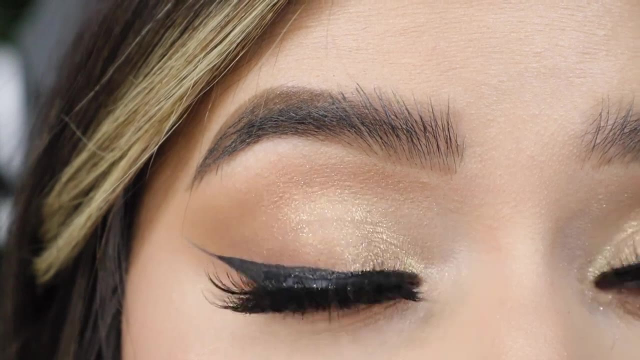 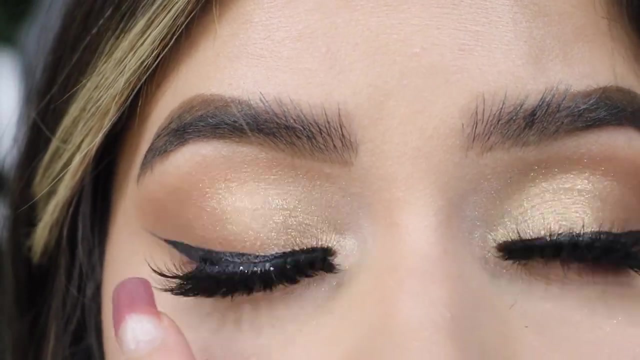 one- samba green is definitely has more of a closer pupil hole where the hydrocore has more of a kind of open detailing to the color contacts. i don't know if you guys can see that through the camera. this is a three month duration and this is a yearly, yearly duration, so there is a huge. 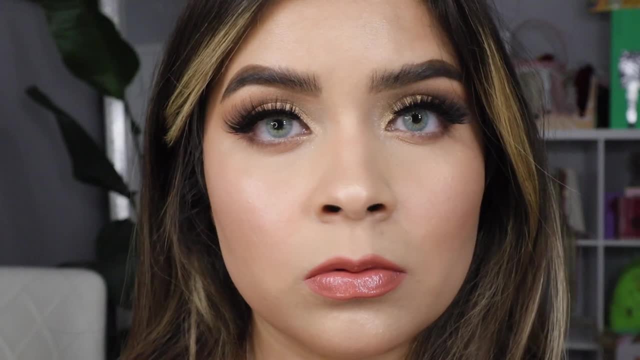 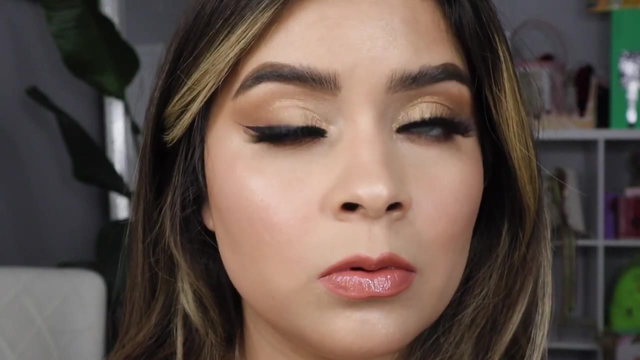 difference between both of these. both feel really really soft. they're not irritating. so i feel like the capacity for the hydrocore iponema is really really good and i really like the color contacts. hydrocore rio iponema- they have really really making them more thinner to the point where it. 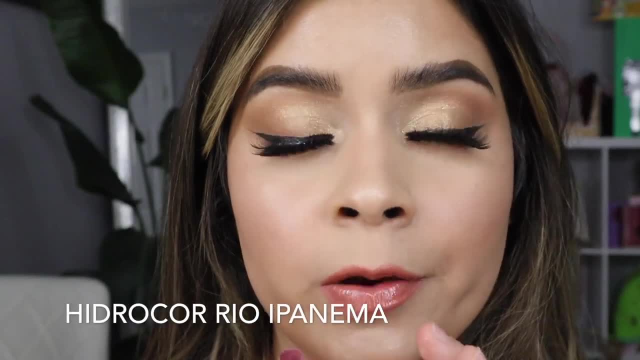 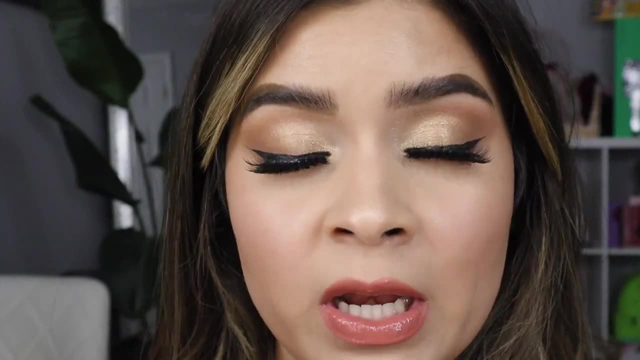 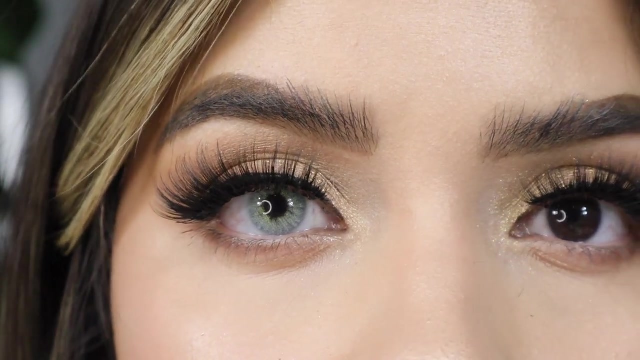 does not irritate your eye. i have the hydrocore rio iponema. just by itself. as you can see the coverage of this hydrocore rio iponema: it covers your dark brown eyes so perfectly that you won't even notice that it is a color contact of both of the hydrocore rio iponema. so 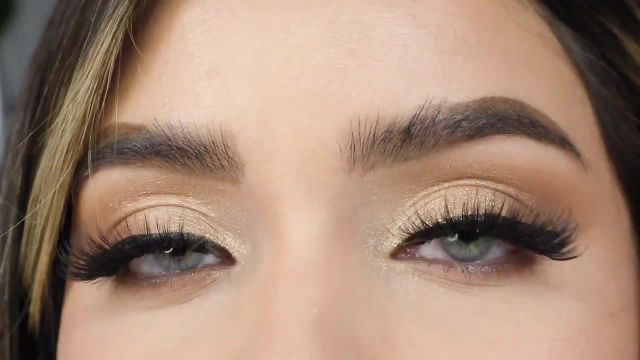 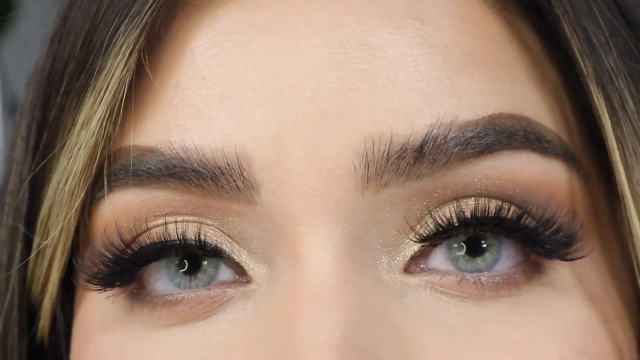 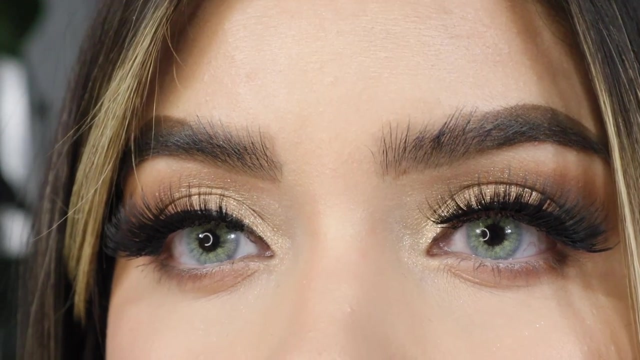 it is definitely, really, really beautiful. i feel like it is perfectly matching with my skin tone and it makes it look surreal on how this color looks. so i really like how solatica created both of these color contacts because you can choose between different durations and you they also carry. 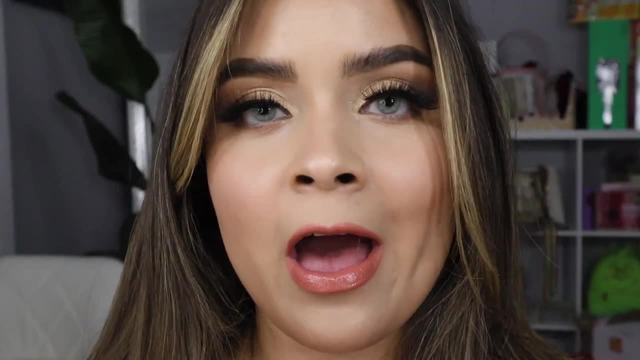 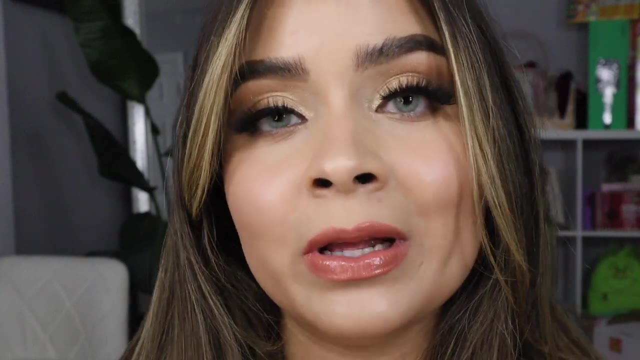 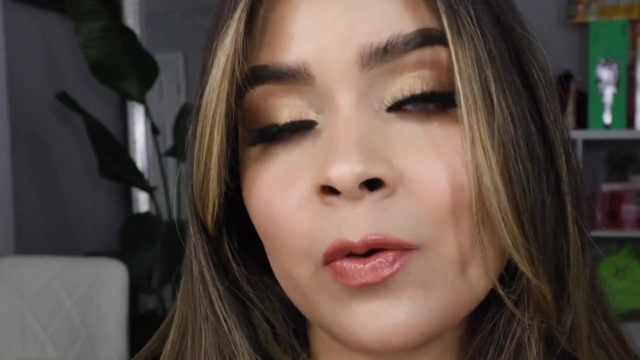 prescription color contacts. for you is the little suma of how the hydrocore rio looks like. i really like both of these color contacts. they look really, really familiar but you can tell like, the difference, like i mentioned by the people whole hydrocore rio, iponema. it is more of a detailed 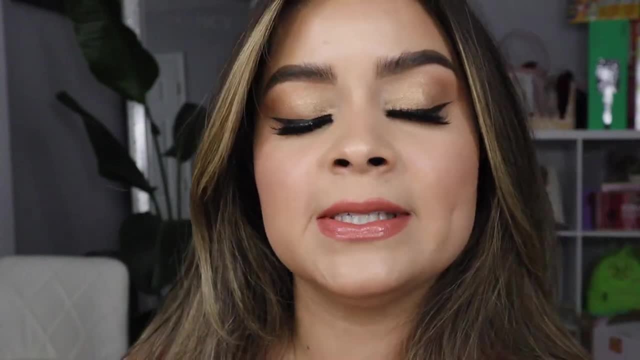 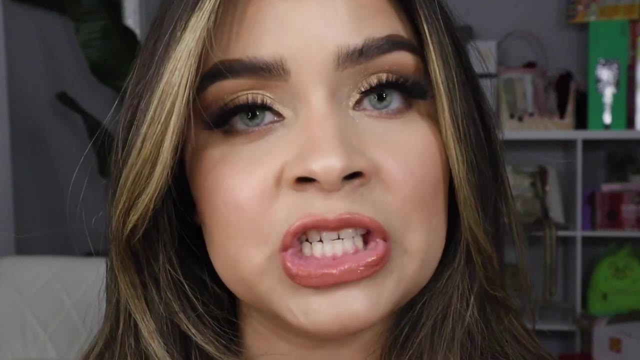 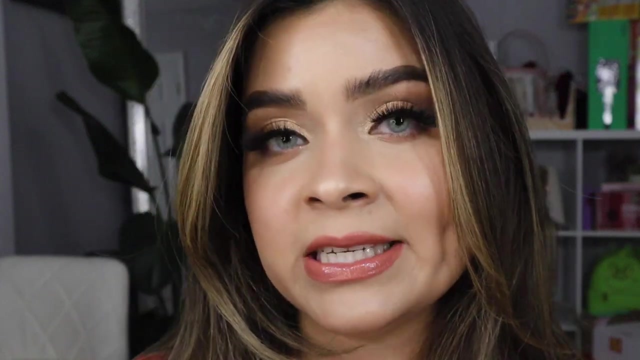 kind of closed up people hole that's on these color contacts. i feel like they look so familiar both of these, but the difference is is the duration like really soft and hydrated? they don't bother my eye at all, as you can see. they're not red, they're more irritated on my eyes. i feel like both of these lenses are really beautiful, so i